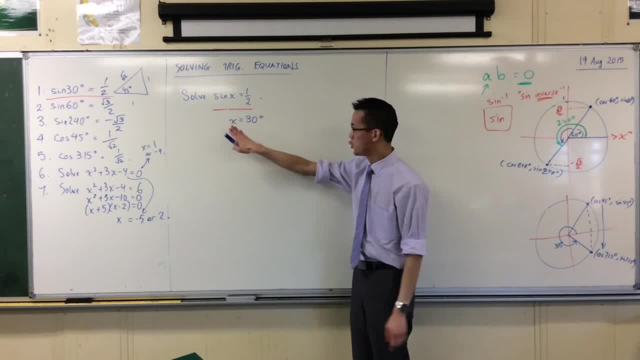 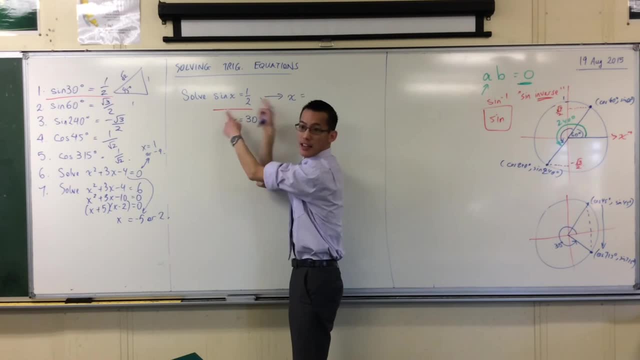 So, being that I want to use sine inverse here right To confirm this result, I can try this. I can write this down and then I can pop it in my calculator. I'm going to do sine inverse to both sides. 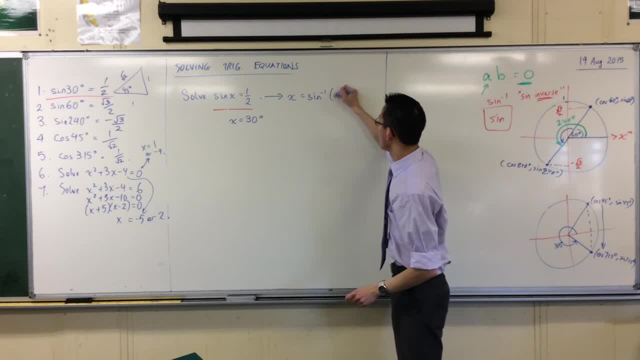 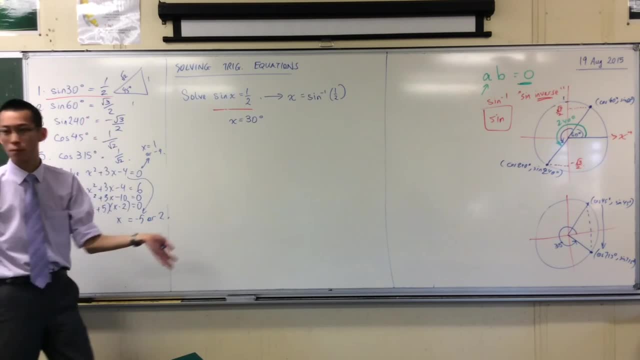 That'll get rid of sine here and it'll put sine inverse over here on the right-hand side. okay, This is just like if you had an equation x over two. you multiply both sides by two, No big deal, Same thing to both sides. 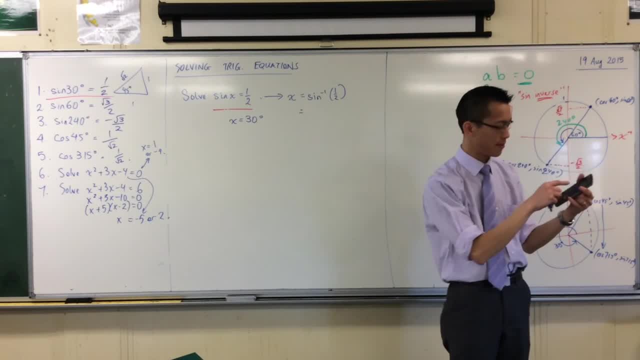 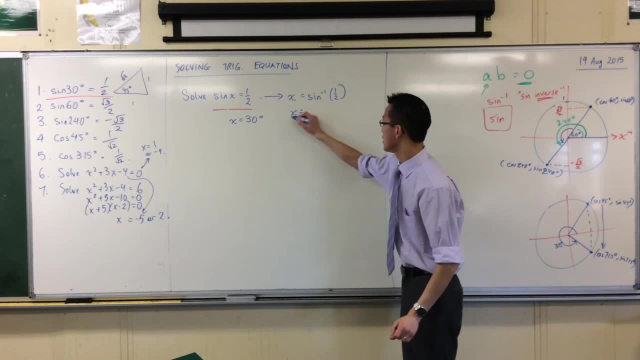 Now go ahead, test it out. Go to your calculator, press shift sine, shift sine and chuck .5 in there And sure enough, right, it tells you. yeah, you were right the first time. x equals 30.. 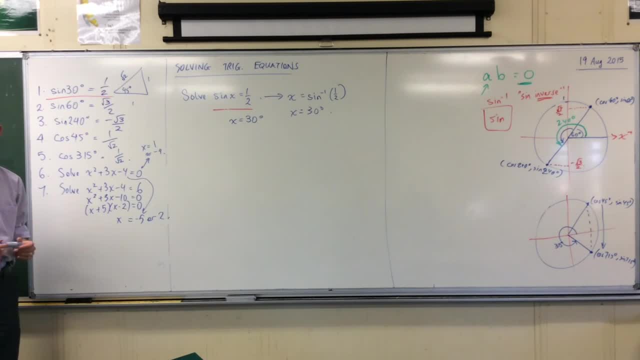 No big deal. The only problem is it's wrong Kind of Okay. so let me explain right. 30 degrees is one of the answers. I mean you told me that right at the start of the lesson. okay, 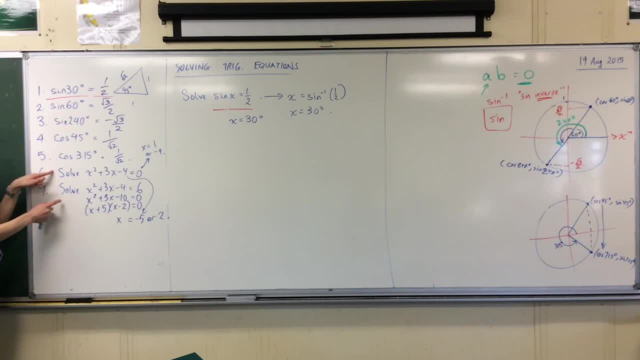 But it's not the only answer. You see these questions here, right? Remember how I was like: oh, I'll test out minus five and it'll work. okay, I put it in. it checks out. okay, But I can also put in two quadratics, right? 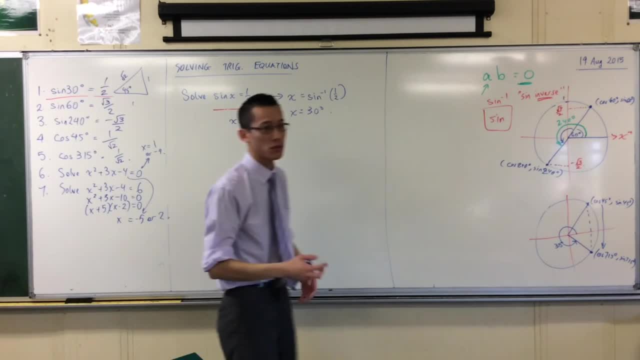 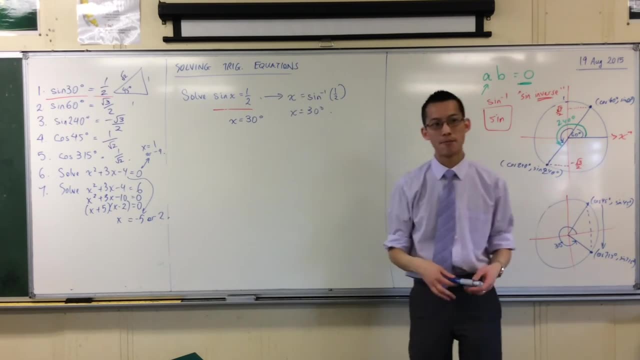 Quadratic equations. They have multiple solutions. They usually have two right Trigonometric equations, just like quadratic equations. they also have multiple solutions And to prove it to you, I'm going to ask you to go back to where you were doing this. 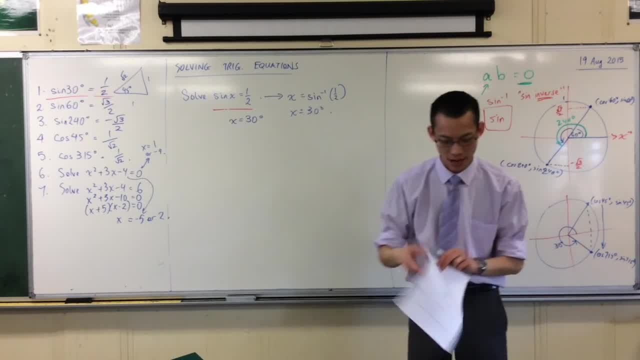 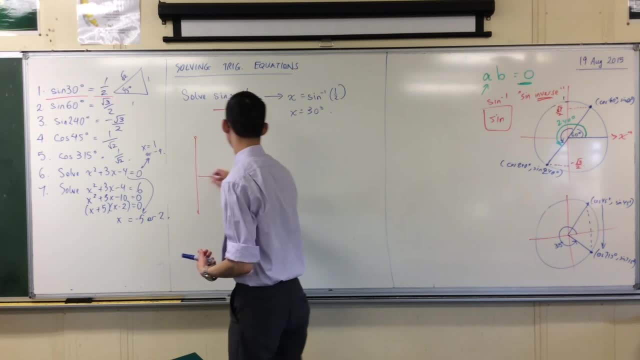 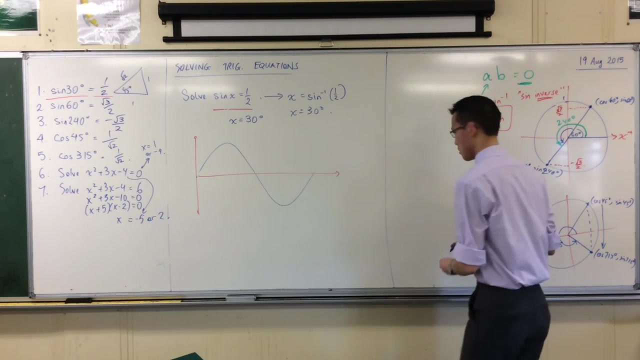 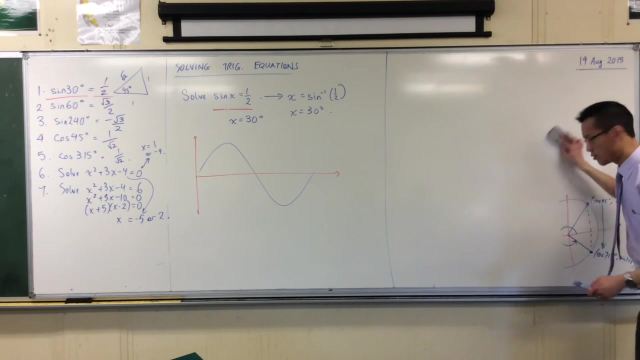 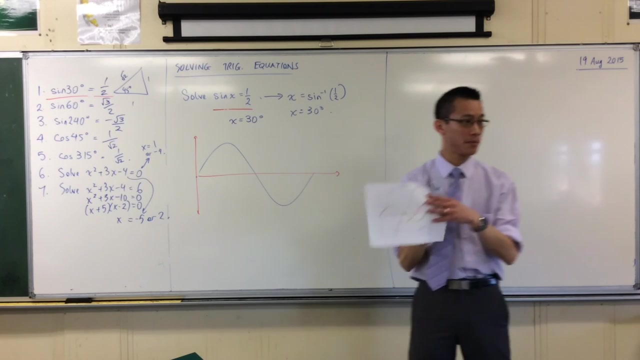 You got all those graphs there. Can you turn back a handful of pages, however many it is for you, and go to those graphs, Okay, Okay, now, once you turn there, I actually want you to take this sign graph and it is worth. if your sign graph doesn't look like nice and clean, like if there's extra stuff on it, like, say, this one. 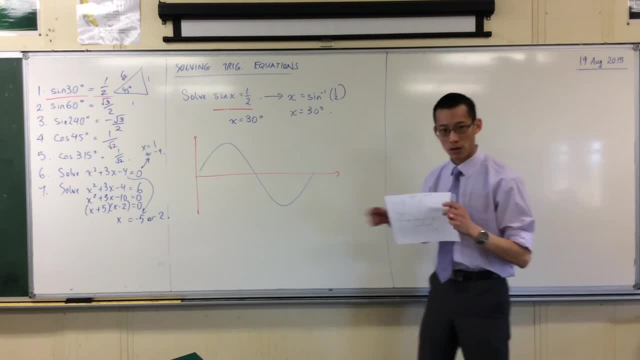 See how I've got lots of extra stuff on there because we were trying to graph tan on this one. I want you to take your graph and make me a little copy on your fresh page based on what you've drawn before. Okay, 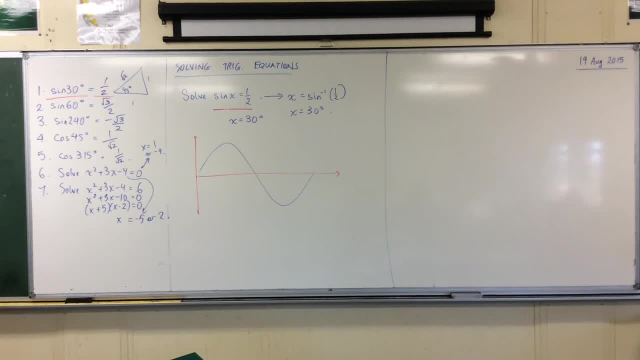 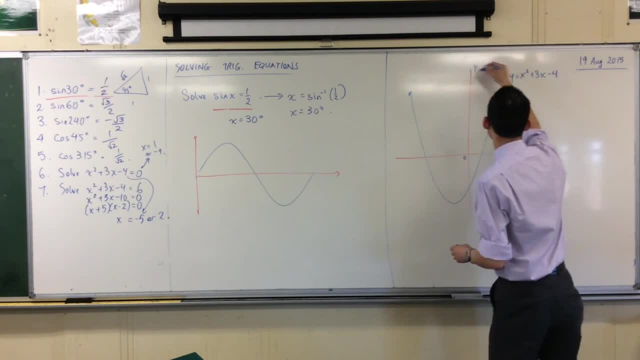 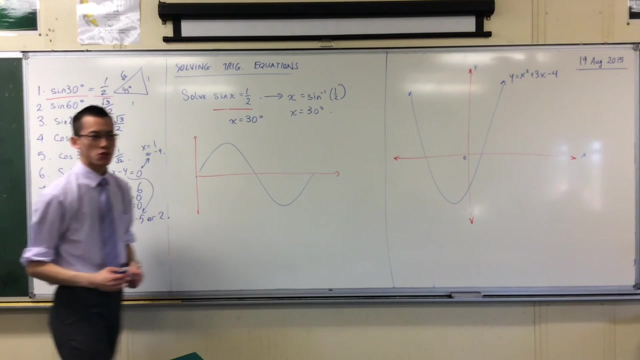 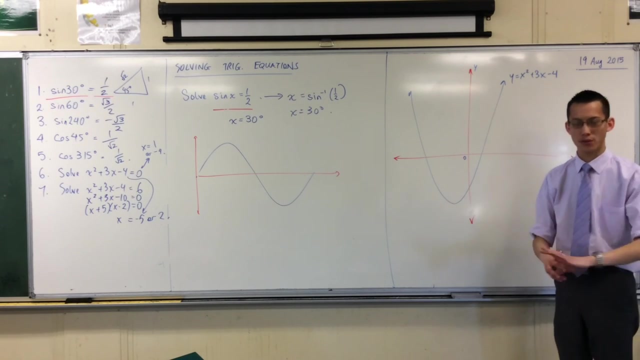 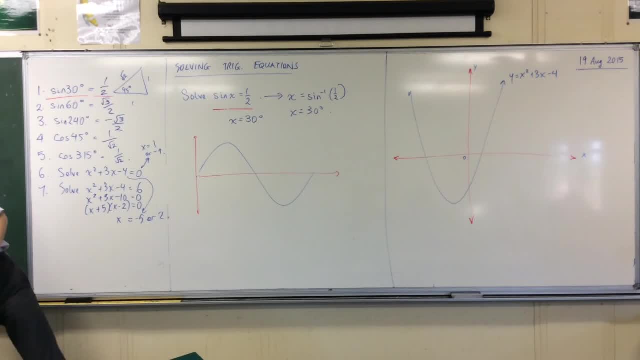 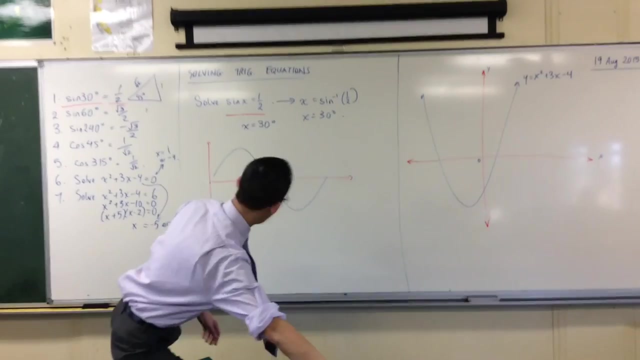 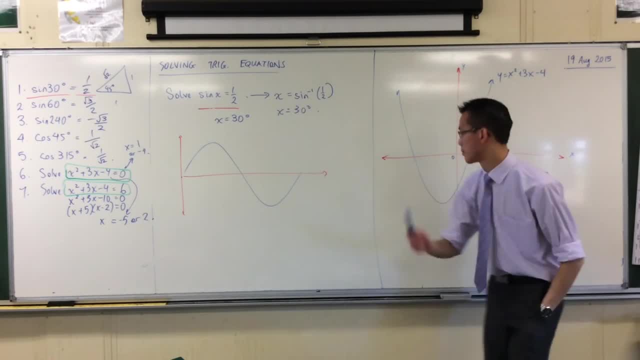 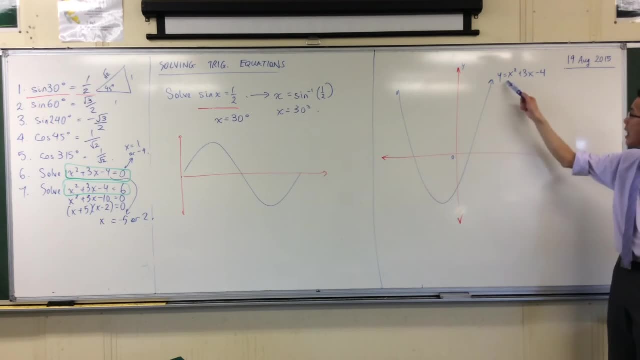 And then the same thing. Why did I do that? Because I wanted to illustrate something. This is my graph of: y equals that same quadratic that you were solving and working with before. okay, x squared plus 3x minus 4.. Now, how do I know? it looks like this: 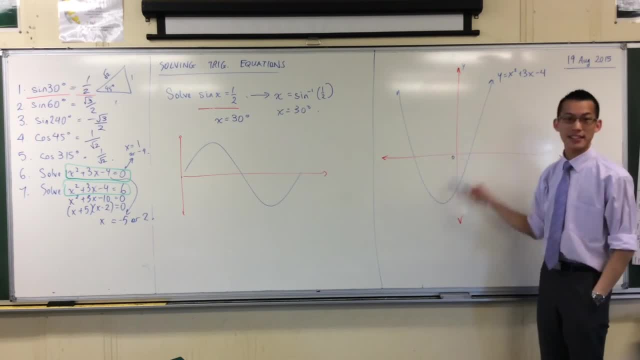 There's a few things I can say. Number one: can you see? this is a smiley. it's a facing up parabola. It's not a facing down parabola. How do I know? There's a single number that tells me it's going up, not going down. 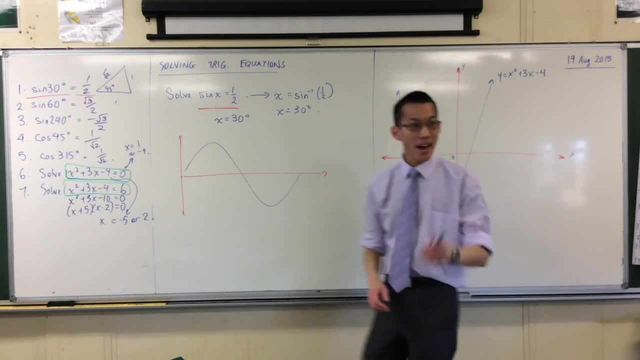 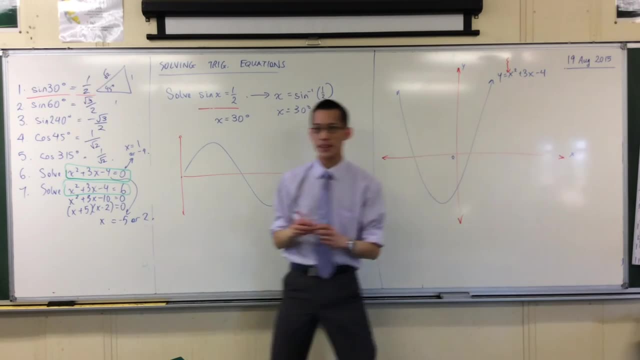 Can anyone tell me which number it is? It's because there's a plus. The plus I'm interested in is one that's actually hiding. It's the one in front of the x squared. right Now, when you write a number like 7, we don't say, oh, it's plus 7.. 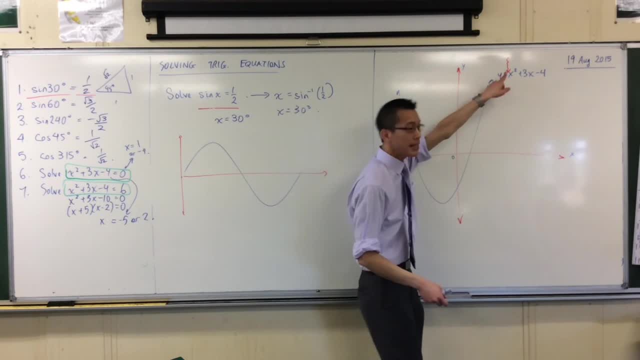 You kind of assume it's positive, right, So nothing is written there, but there really is a plus sign there. If I wanted this thing to be facing down, there'd be a minus sign there, And then there isn't. okay. 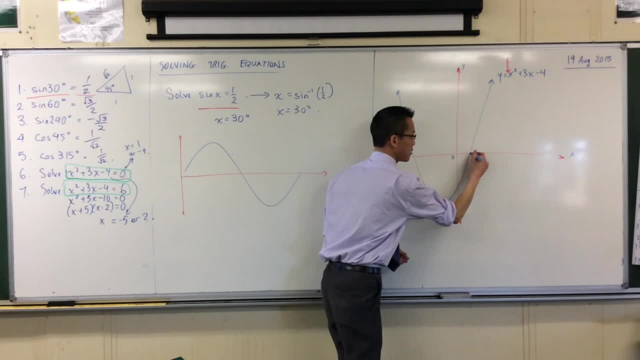 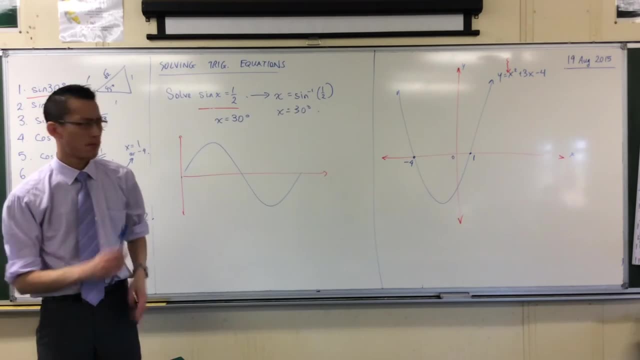 So it's going. It's going up right Now. I also know that I've got this point here and this point here, which are 1 and negative 4.. How do I know that? How do I know that those are the values where it hits the x-axis? 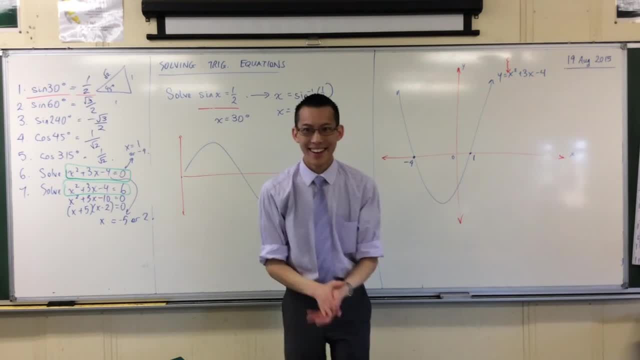 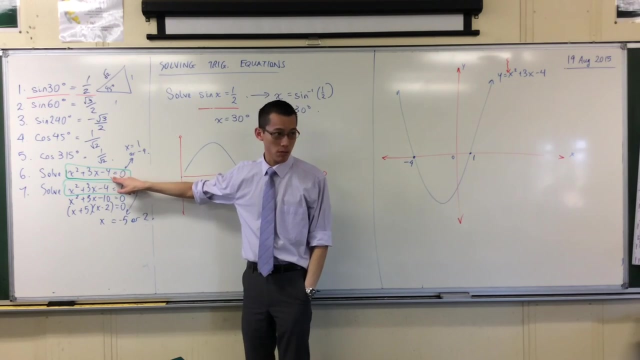 How do I know? those are the intercepts. I know because you told me: right There, it is right there, You factorized it. You factorized it And you told me: x squared plus 3x minus 4.. So the graph: it's equal to 0 at these points. 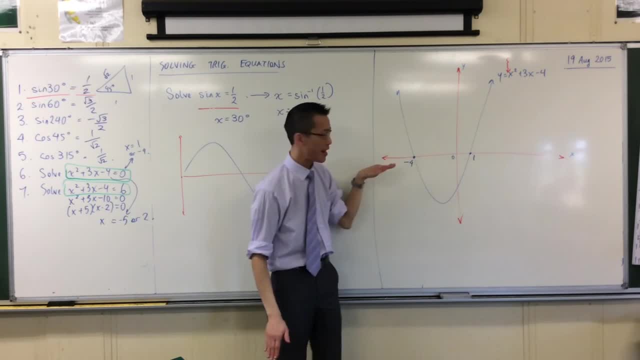 Where's 0?? Here's 0, right. There's the x-axis, right. So at x equals negative 4, and x equals 1, the graph is equal to 0, okay. Another way I could say this is like: the coordinates of these points are minus 4, comma: 0, right. 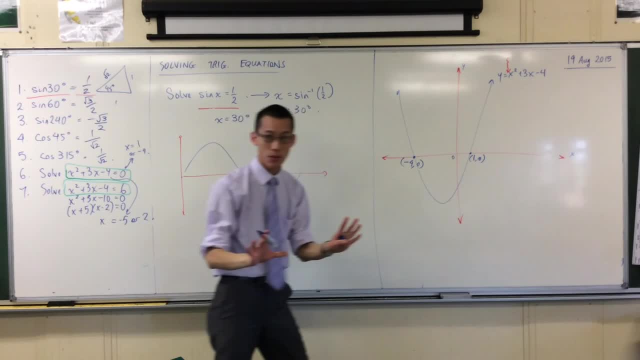 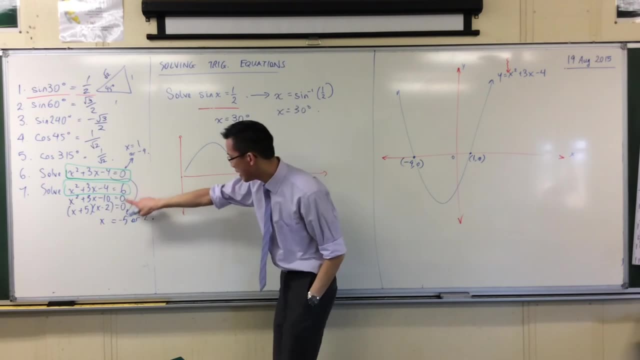 There it is. It's equal to 0, and 1, comma 0,. okay, You happy with that? Okay, Now, how about look at this next equation, right? why did I write it like this? why not just give it to you in this form? 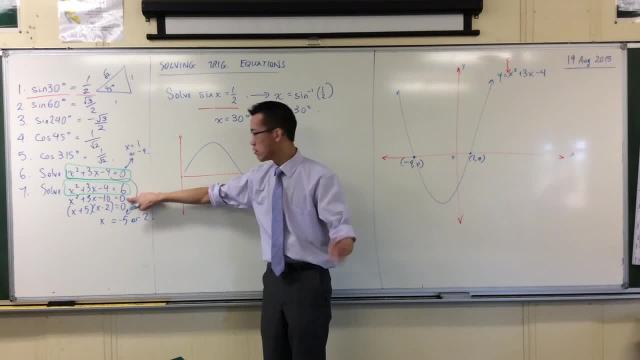 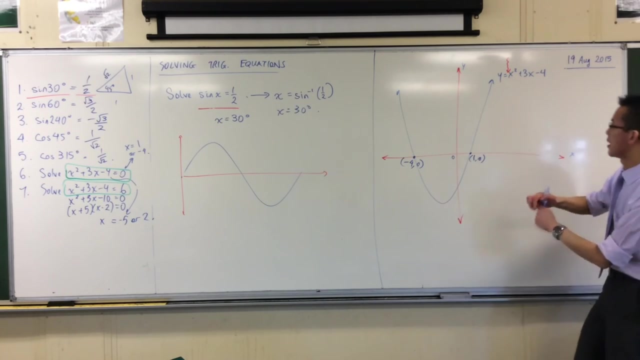 because that's the one you can factorize and then solve. okay, I wanted to show you there's a relationship between these. if solving this gives me these two values, right then solving this will give me a different pair of values. it'll give me- let's see with my scale- 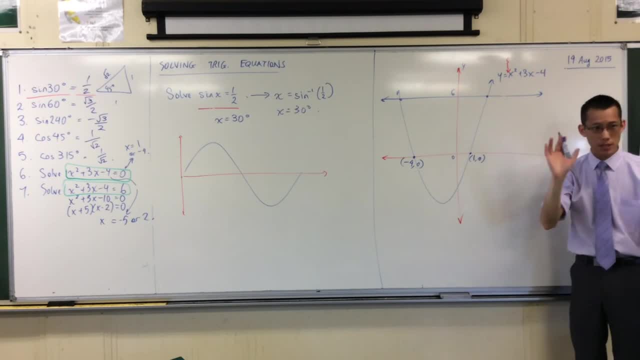 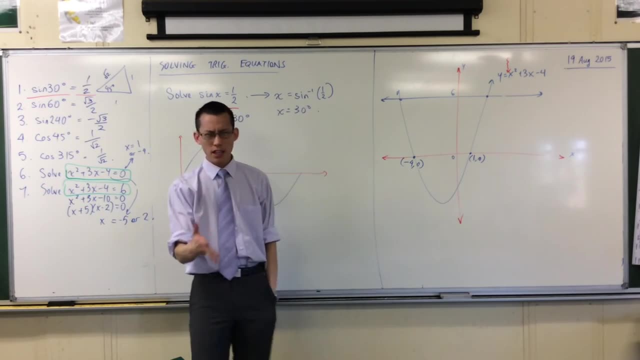 these two values up here. let me see if I can get this across to you right. when we say, would you please solve this equation for me, would you solve this for me? you're thinking about it as what values of x can I put in, and it'll work and 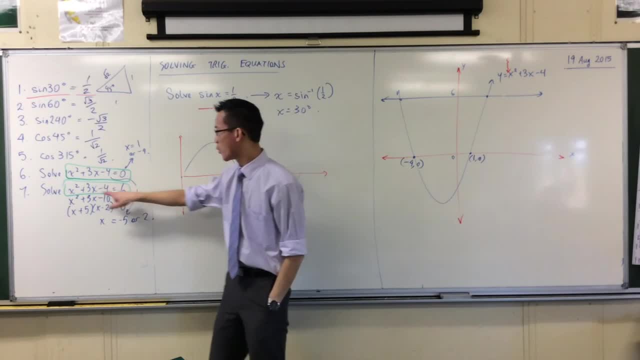 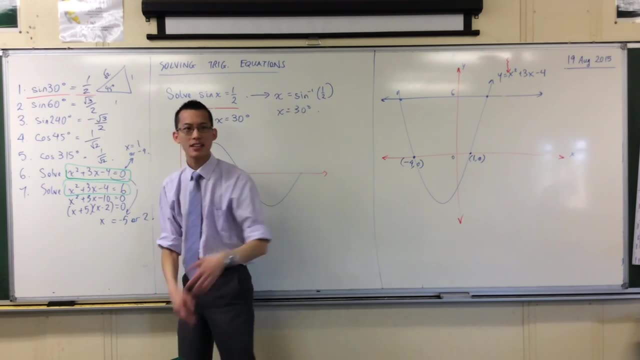 that's fine, that is true, okay, but it's more than that right when I say: solve. what you see on the left hand side is a graph. there is right, what you see on the right hand side is also a graph. it's the x-axis. y equals. 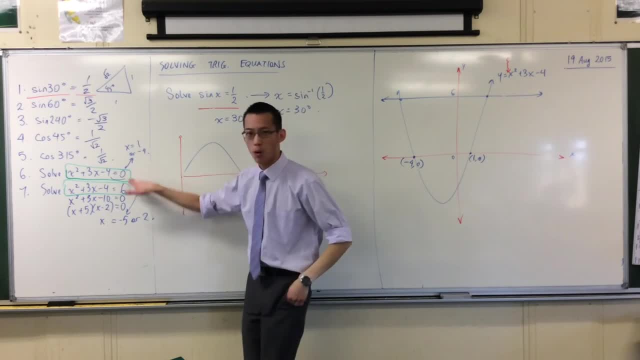 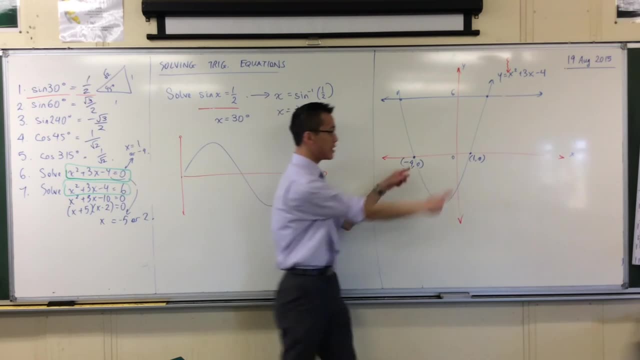 0. right, and what I'm looking for when you solve is tell me where they collide, tell me where they intersect, tell me where they're equal to each other, right? so these happen to be the two places where that graph and that graph are equal, right? so when you go ahead and solve this question,